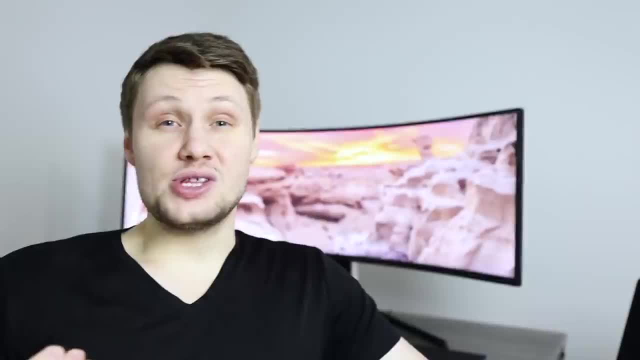 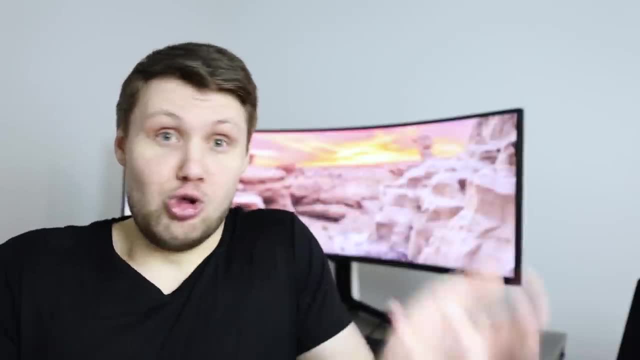 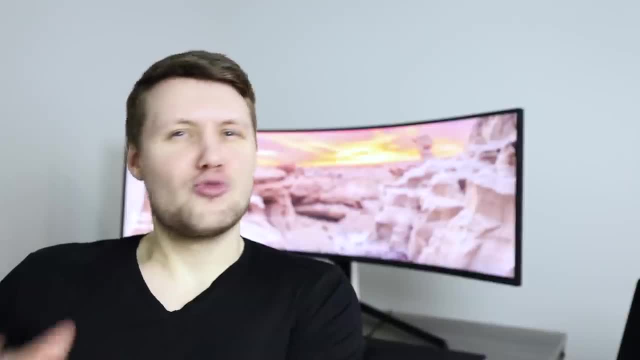 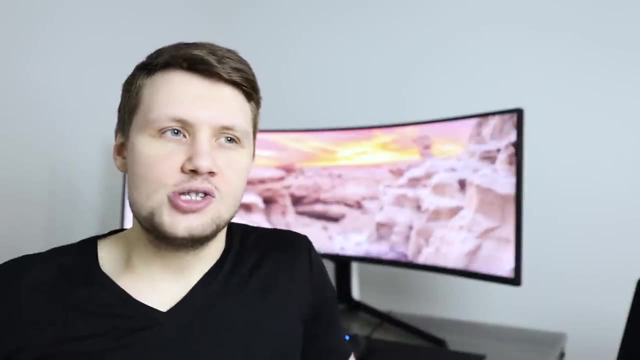 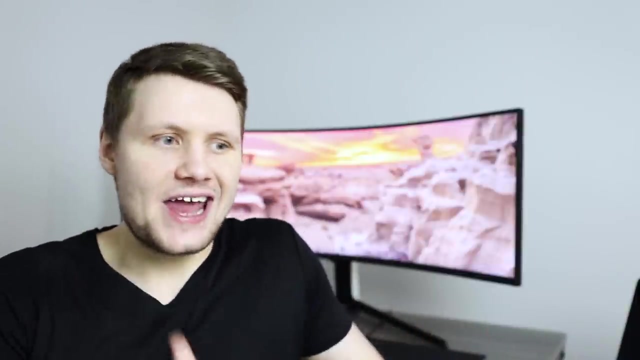 of a tool that you're using on your job but not necessarily like your primary function. if that makes sense And if you answer no to some or most of these- you know sub questions- well- then maybe machine learning isn't for you. Similarly, if you're strongly considering getting 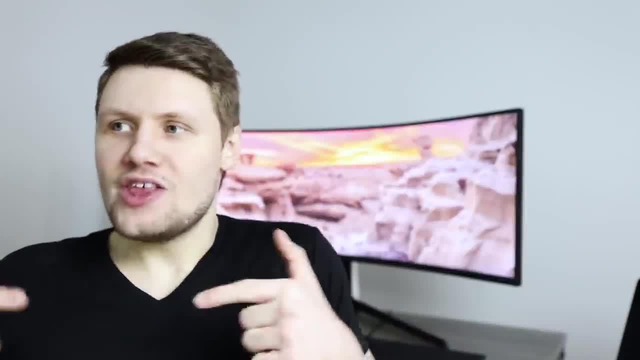 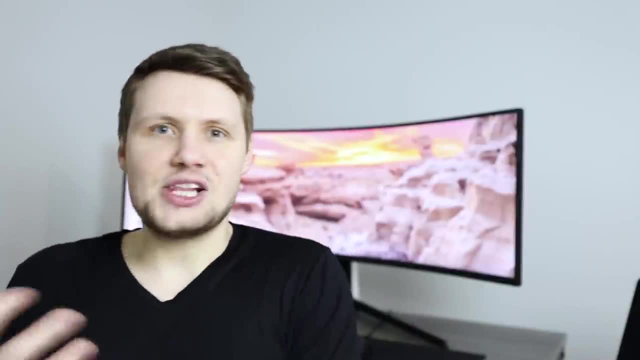 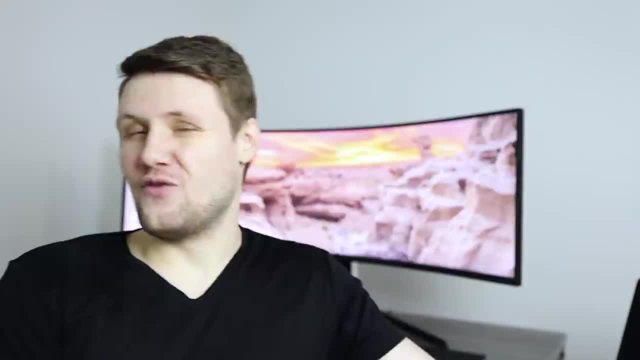 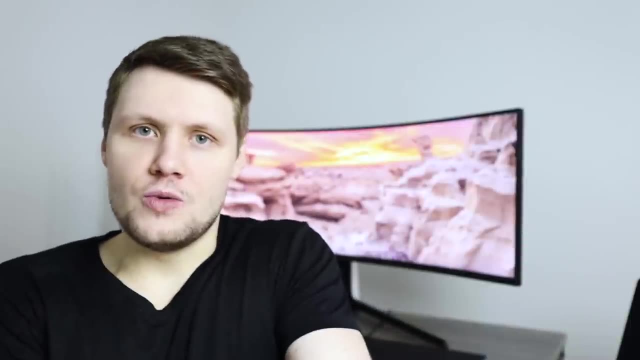 well then, maybe backend or infrastructure aren't really for you because they're a bit more invisible, and maybe front-end engineering or mobile engineering is going to be more relevant to you. So that's the first question that you have to ask yourself. The second question: 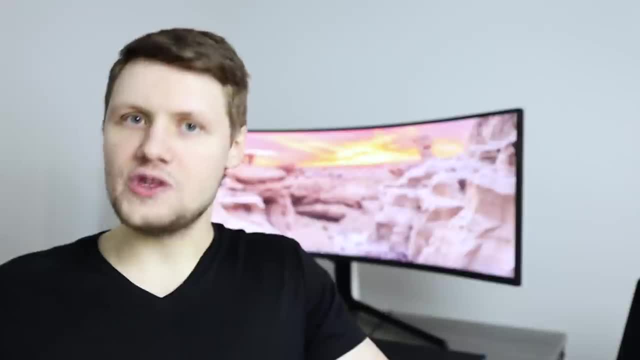 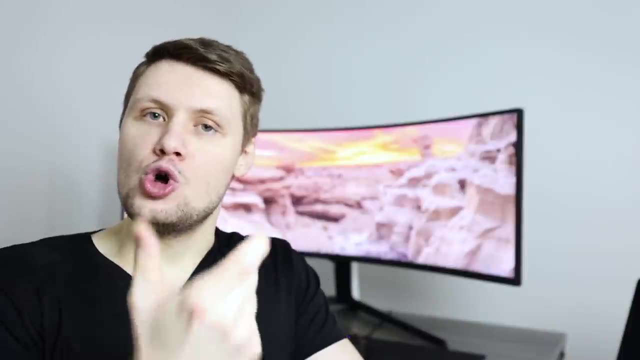 is a little bit more nuanced, but basically you want to look at all the specializations, or at least the ones that you haven't eliminated yet, And you want to look at what the typical work that someone in that specialization does. I'm not talking about the most exciting. 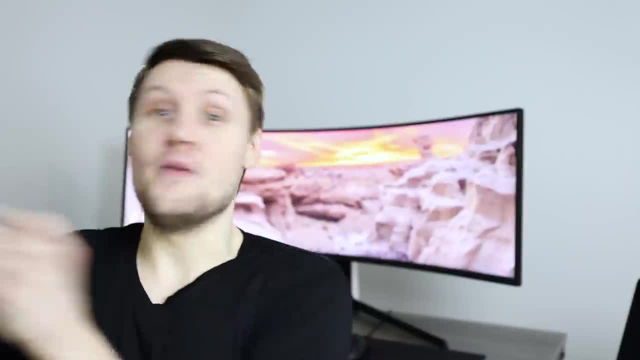 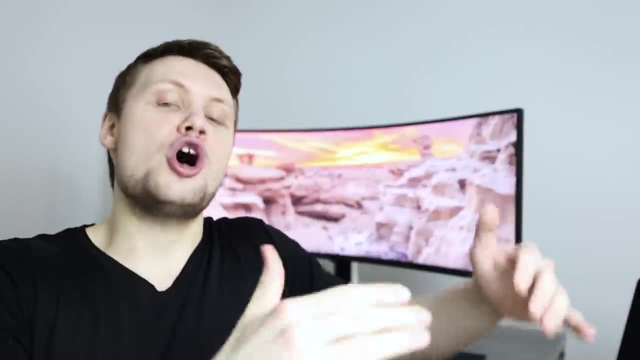 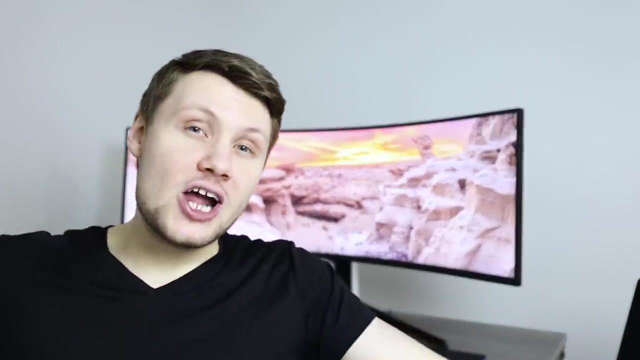 you know 5% or 10% of work that a machine learning engineer or front-end engineer does. I'm talking about the 80%, the 90%, what they do on most days, because I think that it's very easy to be seduced by the most exciting projects, the most exciting features Like, for example, 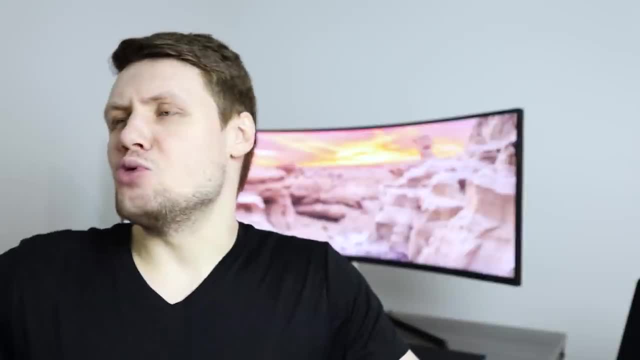 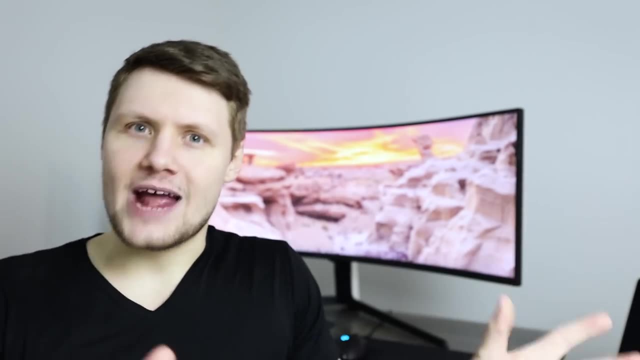 you might think, Oh, I would love to be a machine learning engineer because I would love to work on AlphaGo at Google, the AI that beats you know the world-class uh Go, champion Go being a board game, And that's why you're interested in machine learning engineer. 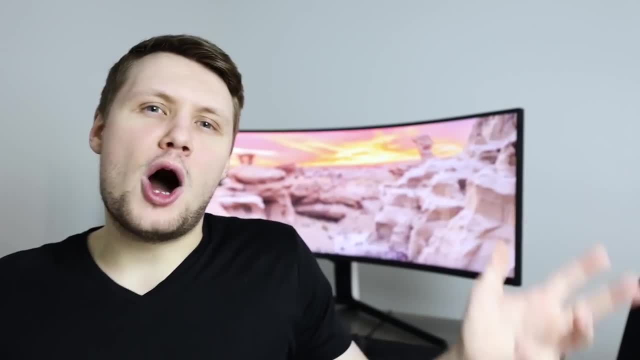 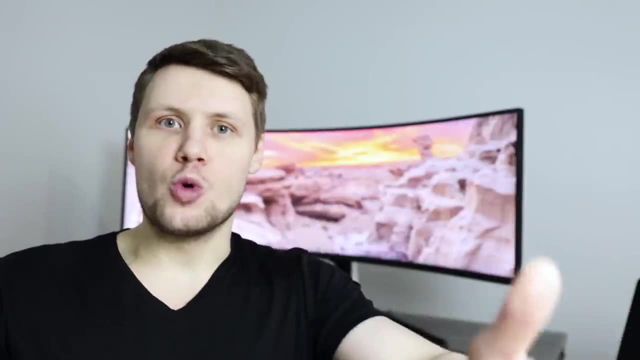 or you want to develop, you know, the most cutting edge ML models at a hedge fund. Or let's say that you're considering front-end engineering and you're really attracted to it because maybe you want to work at AlgoExpert, my company. 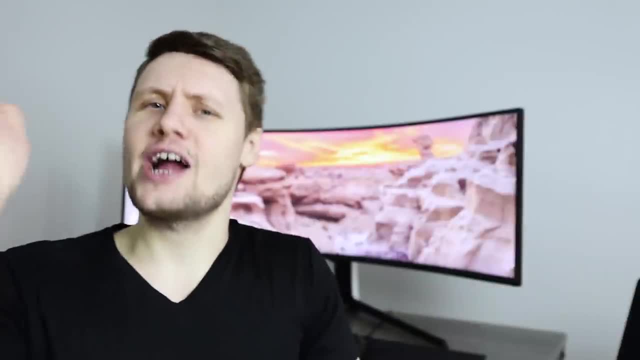 by the way, if you're a software engineer preparing for your coding interviews or systems design interviews, check out my company, AlgoExpert. go to algoexpertio and use the promo code Clem C-L-E-M for a discount on the platform. But you're excited to become a front-end engineer. 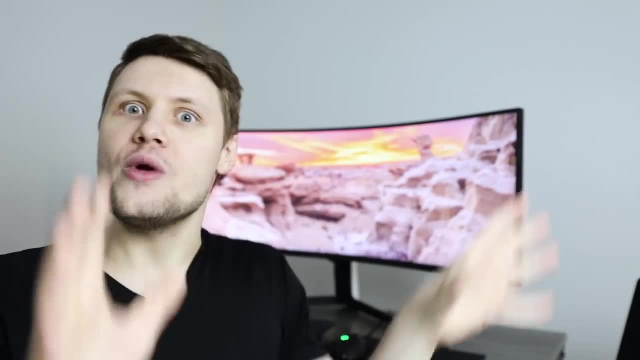 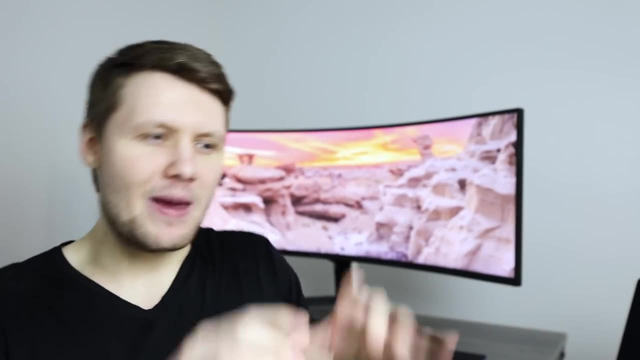 at AlgoExpert because, specifically, you want to work on the coding workspace of AlgoExpert, which is kind of our bread and butter, you know, feature on the platform. It seems really exciting to be able to to write code, run the code, all that stuff. But the truth is that both 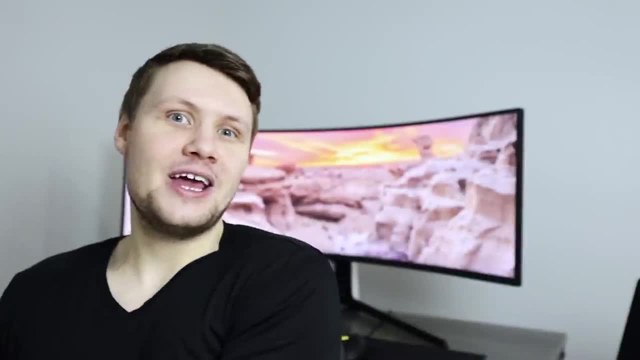 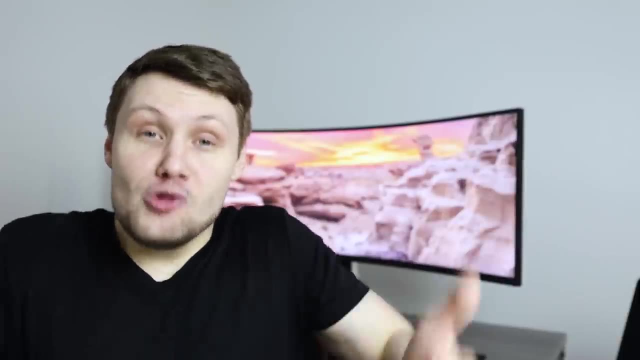 for front-end engineering at AlgoExpert and for machine learning engineering at Google or at a hedge fund. you are likely not going to be working on the things that I mentioned most of the time, if even at all. So you want to look at the stuff that you are going to be working on. 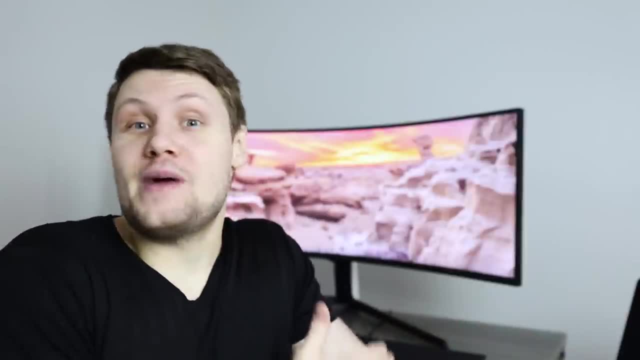 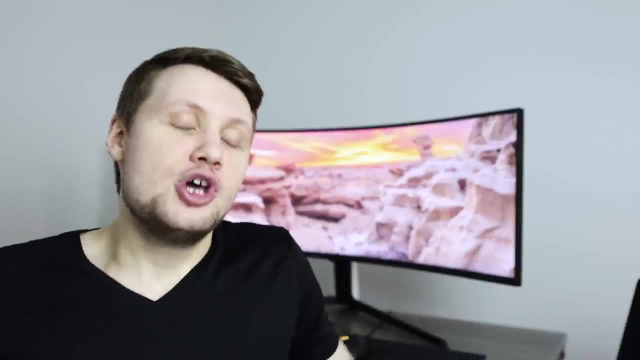 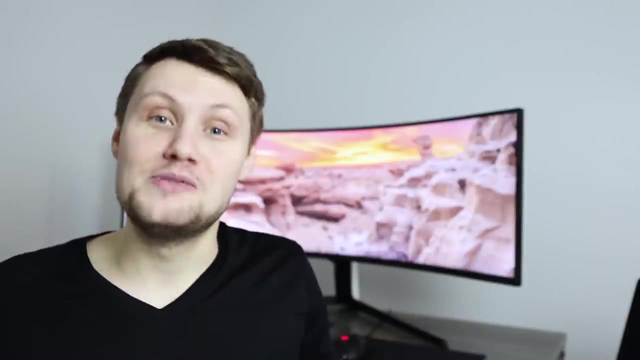 So if you're a front-end engineer, you are likely going to be spending the majority of your time putting forms on a page, or at least that is something that most front-end engineers spend a good amount of time doing. You're not necessarily only going to be doing that, but believe me when I tell you most websites. 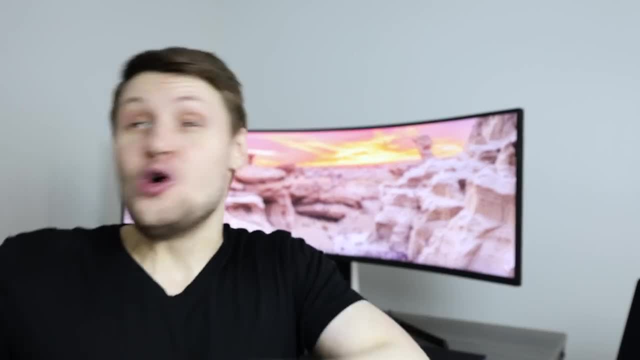 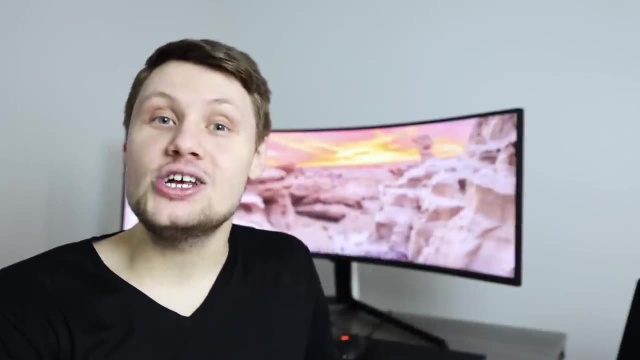 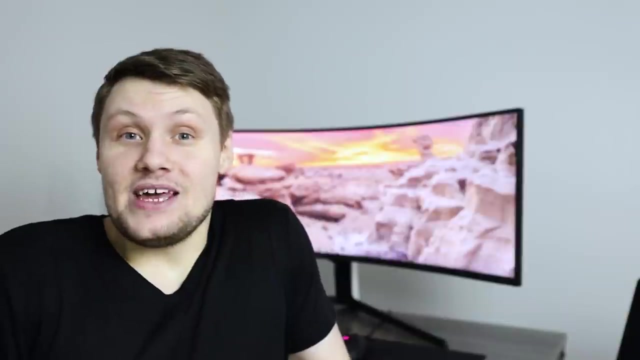 have a lot of forms either, you know, to create accounts or to submit things or to update settings. You have to have forms on pages. That means putting input fields, you know, text fields, radio buttons, submission buttons, and that might not be super exciting. Maybe you do enjoy that. 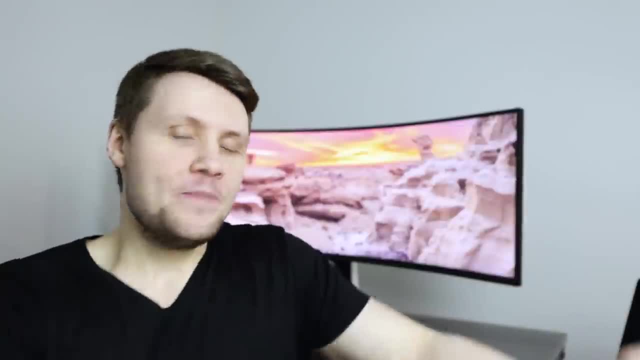 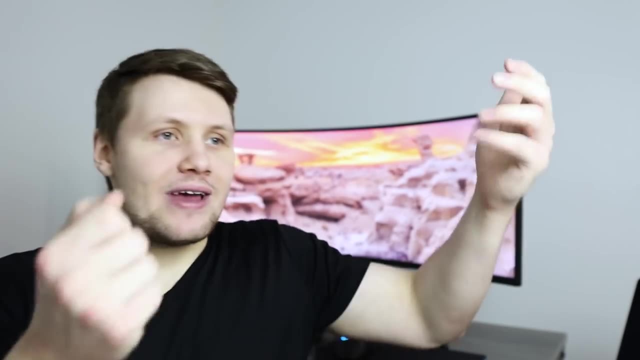 but it might not be as exciting as you thought front-end engineering as a whole would be. Similarly for machine learning. maybe you're going to spend most of your time polishing data sets, figuring out what features in a data set you really care about. 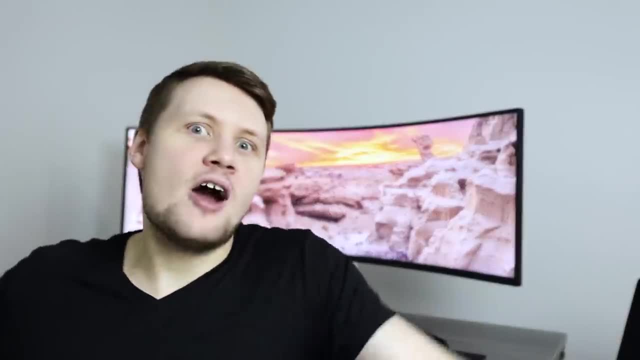 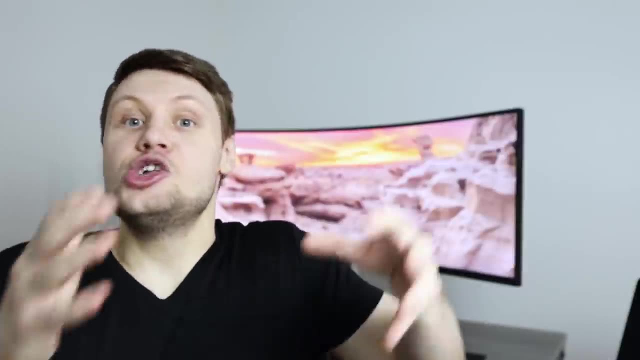 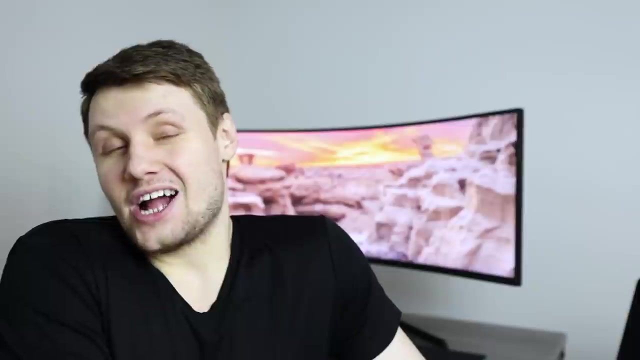 and you're not really going to be spending your time developing cutting edge machine learning models. I'm just spitballing here, but the point is identify what these specializations spend most of their time doing and see if that's something that you could actually see yourself doing a lot or if it's actually something that turns you off. 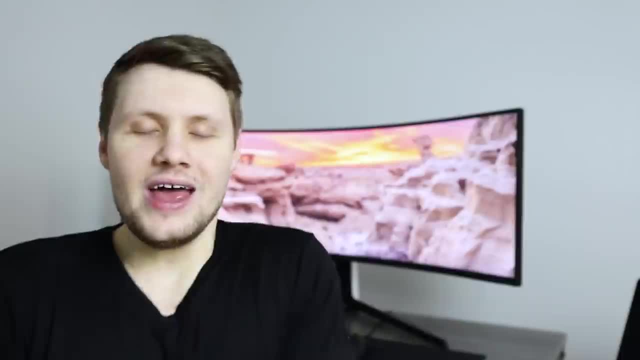 Now. hopefully this video was helpful, but please do consider subscribing to my channel if you enjoyed it. I would love to keep up with a new video every week. If so, feel free to hit that like button. question that you have to ask yourself has to do with practicality. How practical is it for you to? 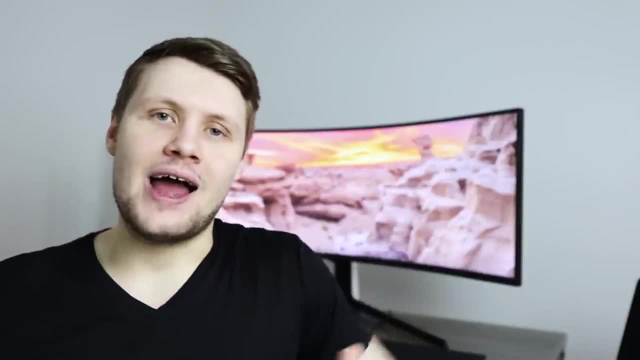 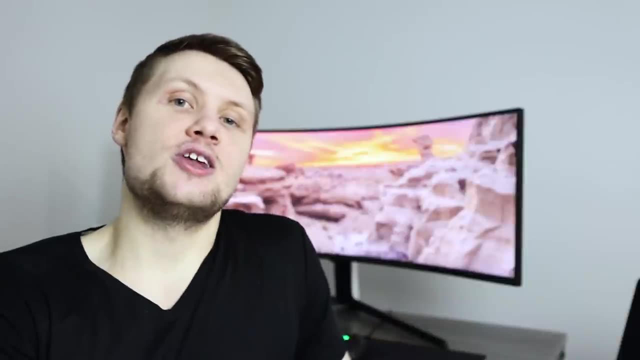 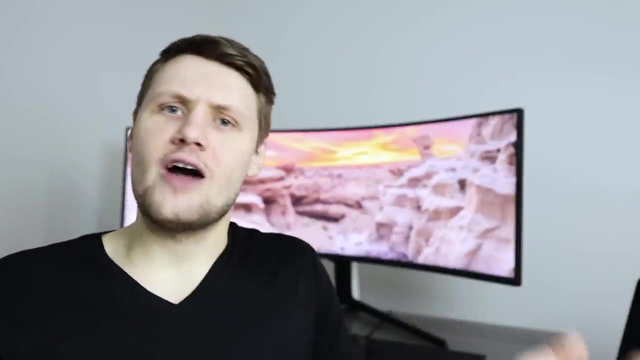 pursue a specific specialization at the current time, given your current situation. So I'll give you a couple of examples where pursuing a certain specialization might not be worth it. Let's assume that you just graduated from a coding bootcamp. you learned full-stack JavaScript. maybe you've 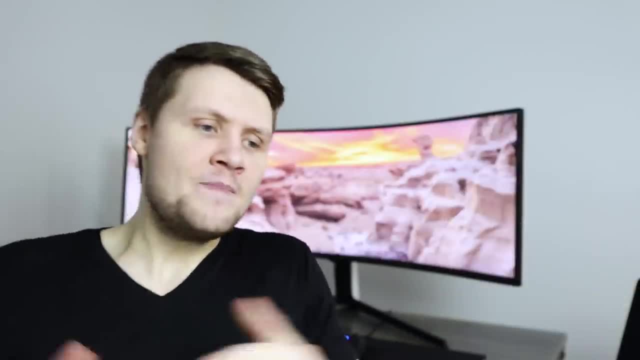 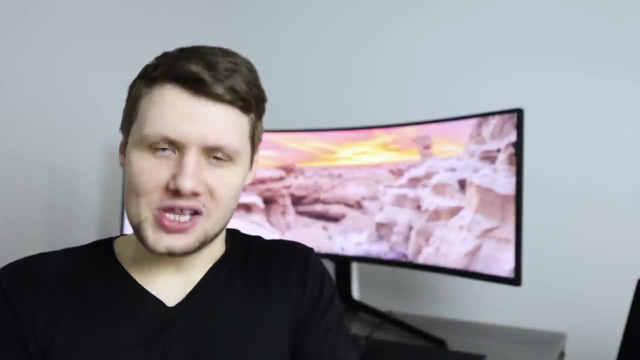 picked up Python by preparing for your coding interviews with AlgoExpert, and you suddenly develop an interest in infrastructure engineering And you're like, okay, I've answered the first two questions that I've talked about in this video. I want to get into infra-engineering, So I'm going. 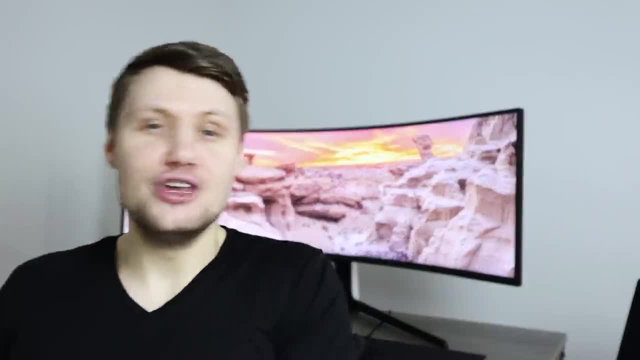 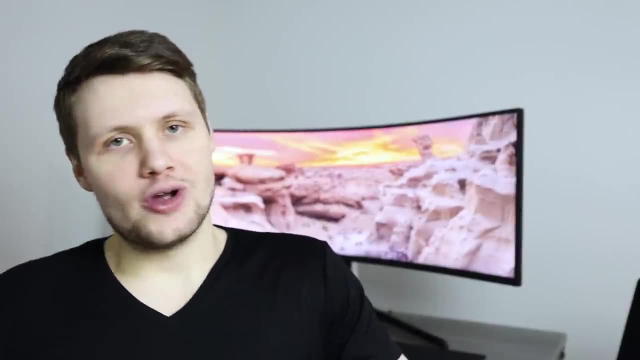 to start learning Golang, if that's what you know. they use as a programming language for infra-engineering, Docker, Kubernetes, all this stuff- and I'm going to apply specifically to infrastructure engineering jobs. Well, practically speaking, that might not be the. 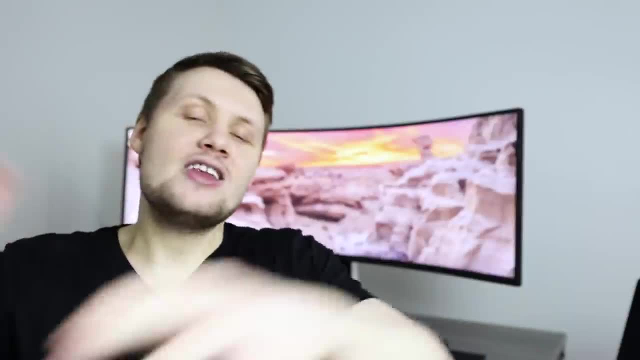 best way to pursue a specialization at the current time, given your current situation. So I'll give you a couple of examples where pursuing a certain specialization might not be worth it, Because you're suddenly going to be learning brand new technologies after you've already spent a lot of time learning a new skill set. you're going to be limiting your opportunities. 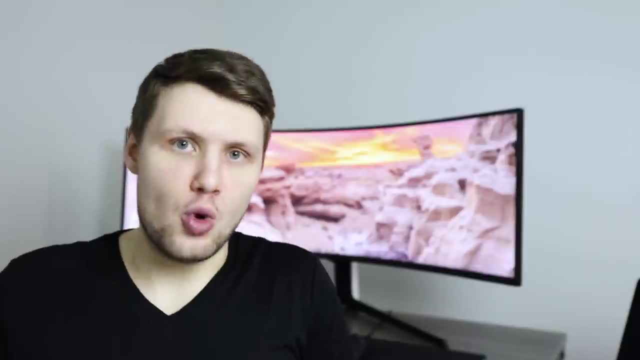 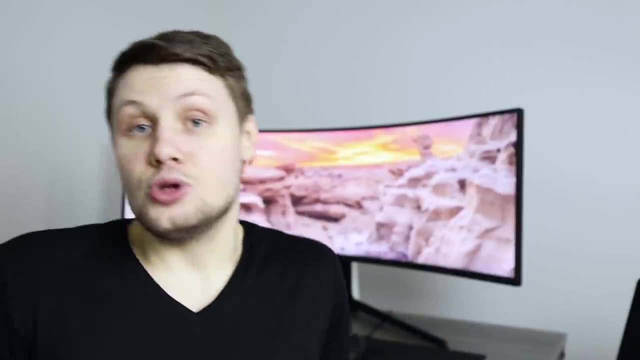 maybe it's going to be much tougher for you to actually get your foot in the door of the software engineering industry, So it might just not make sense from a practical point of view. Similarly, maybe you're a college grad. you just graduated from college with a computer science. 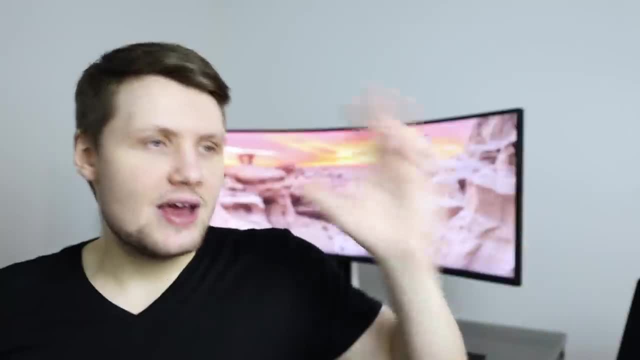 degree and you're about to apply for jobs. but you decide in your mind: you want to be a front-end engineer, you want to be a software engineer. you want to be a software engineer. you want to be a front-end engineer. you will only apply for front-end roles or if you apply to big tech. 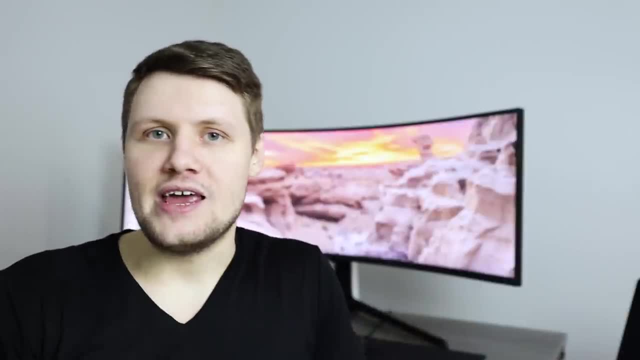 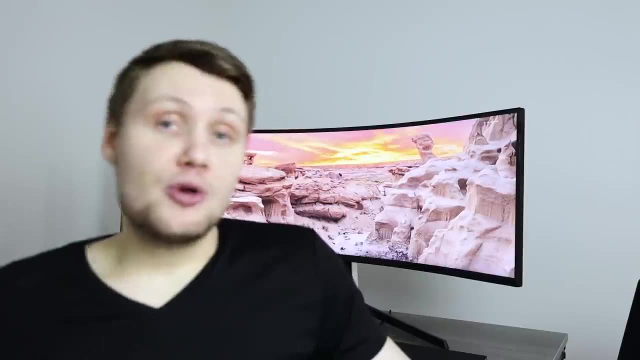 companies like Google and you get in. you're only going to want to match with teams that have front-end openings. Well, that might end up working for you, But you might also be limiting your opportunities And maybe you know you're going to effectively close a door on a back-end 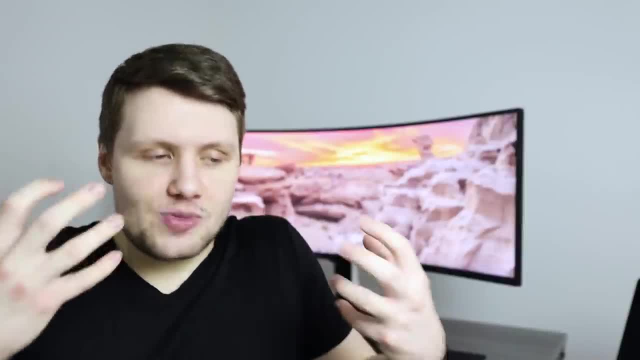 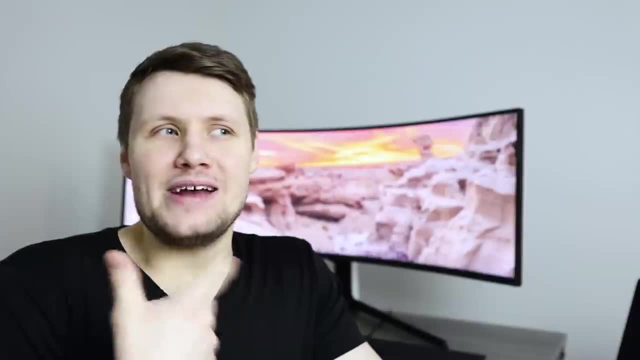 job that you would have gotten, that would have been amazing. just because you think that you really want to become a front-end engineer And at the start of your career, it might not be practical to close opportunities like that. Now don't get me wrong. I'm not saying that you. 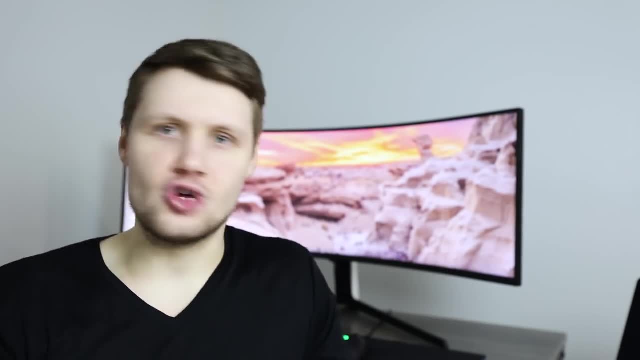 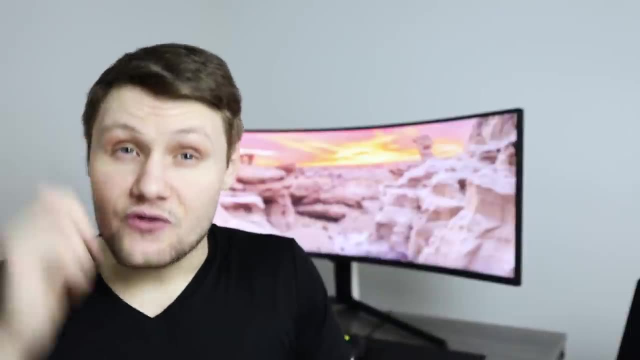 absolutely shouldn't do what I just described of being a college grad looking for front-end roles. Maybe you truly are, like for sure, passionate about front-end. you're really skilled in front-end, and so you don't think that you're going to be closing off that many opportunities. 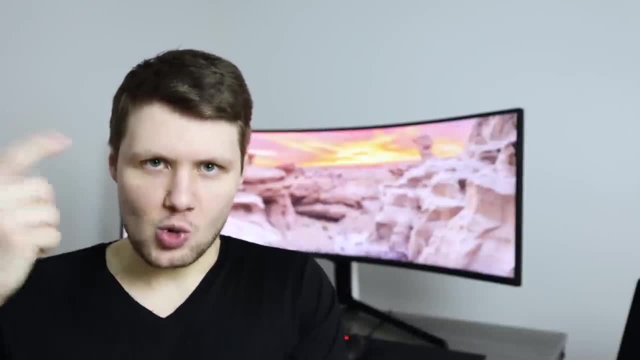 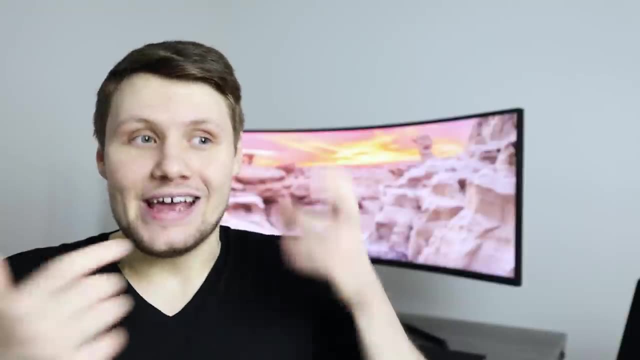 All that I'm saying is that you should ask yourself this question about: is it practical for you to pursue a specific specialization right now? And if the answer isn't a definitive yes, then maybe you reconsider. And as a final point before I finish off this: 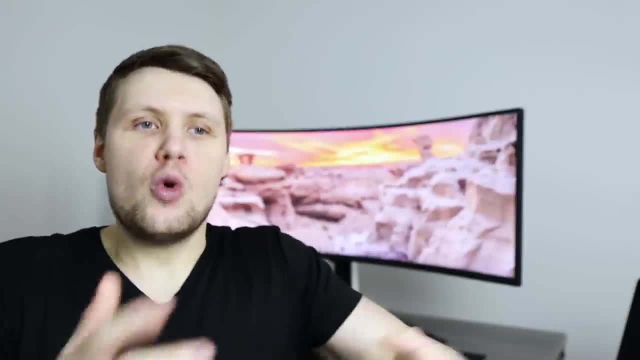 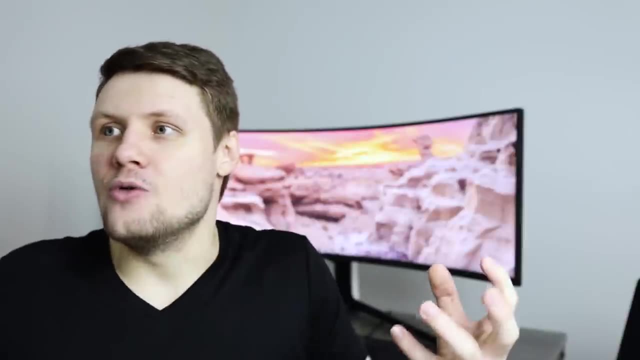 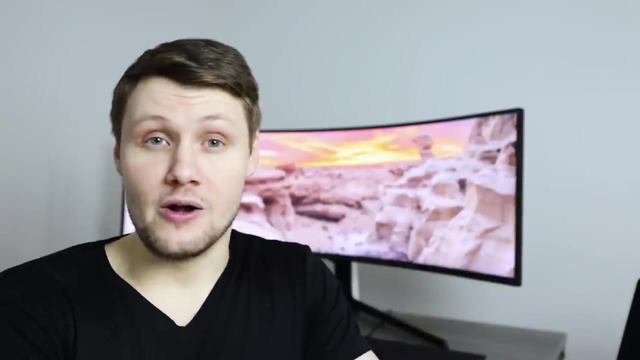 video. I do want to remind you that you are not bound to your very first job or your very first specialization. You are not bound to whatever it is that you do in the software engineering industry during your first two, three, even five years of your career. In this day and age, you can always. pick up new skills, especially in tech. You can learn new skills, expand, switch to other specializations after self-teaching yourself the specialization that you want to switch to, even coming from another one. So don't feel like this is the be-all, end-all decision that you have. 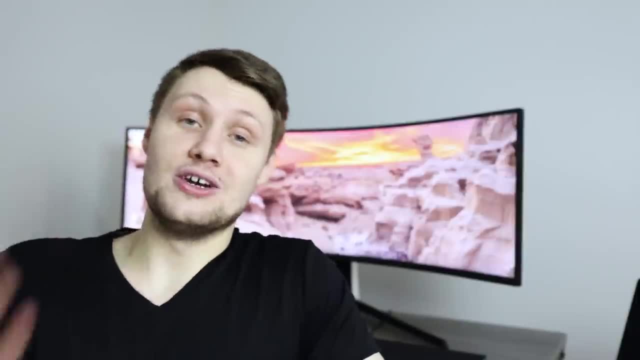 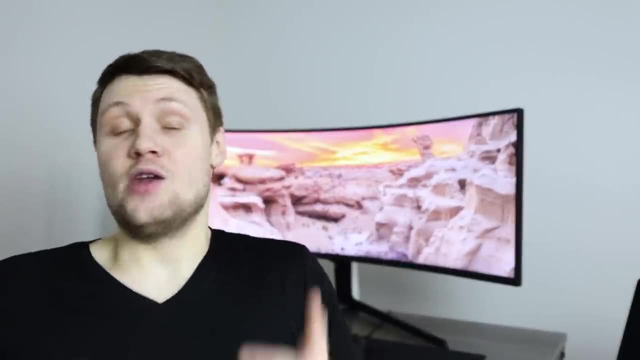 to make As a good example. one of my former co-workers at Google had been a front-end engineer for like five years Before Google at Google. he was really good at Angular CSS and while I was at Google with him, he realized that he was going to have to do a lot of work on his own, And he 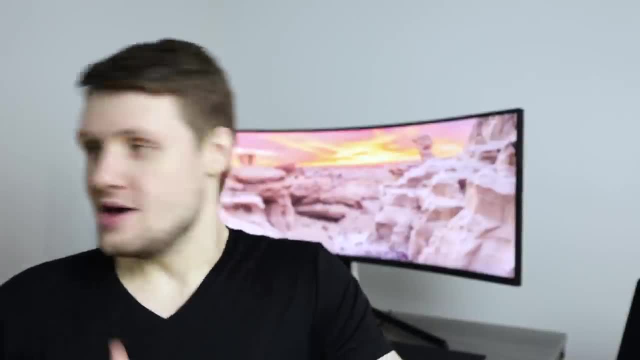 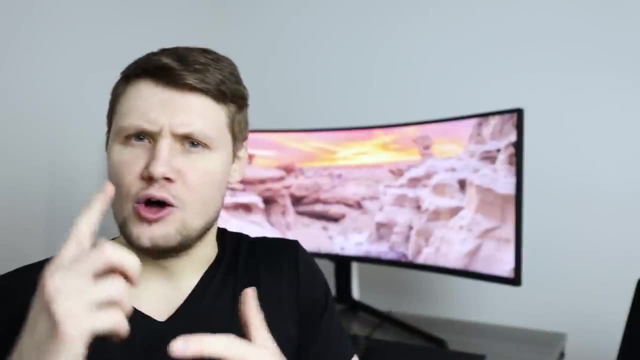 was interested in machine learning And he started teaching himself machine learning at home, using courses, tutorials, whatever. He started taking machine learning classes at Google. I think he even did a rotational program And then by the end of it, he was basically a machine learning. 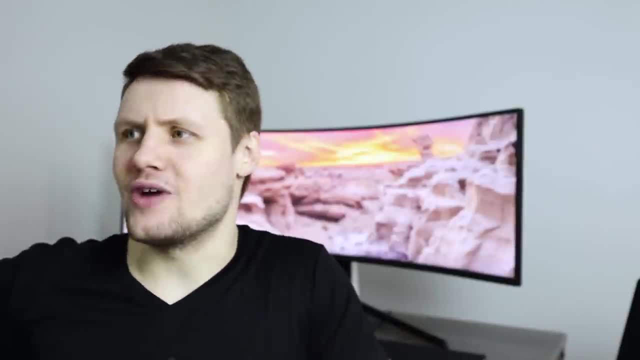 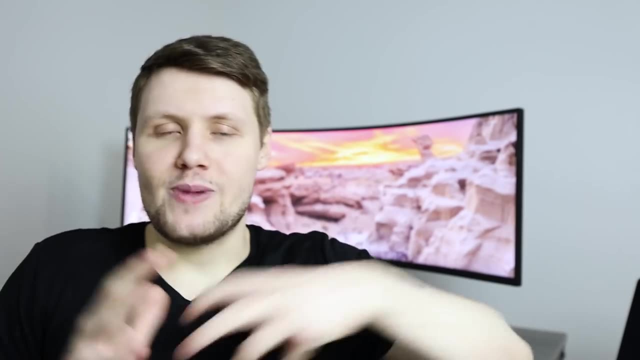 engineer, or at least employable as one, And I think he ended up leaving Google and creating his own company that does something with machine learning, And so that's just a good example of like you can always switch specializations, even from something like front-end engineering to 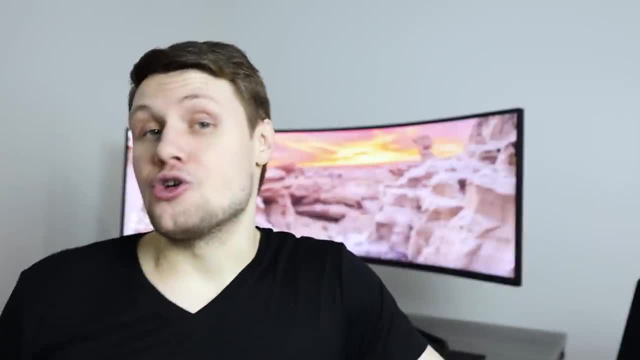 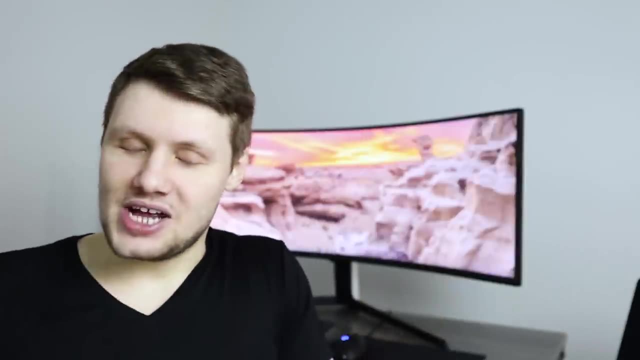 machine learning, which are pretty fun. I think that's a really good example of like you can, far removed from each other, later on in your career. You are not bound to the first specialization that you pick, So hopefully you found this video insightful. If you did, please don't hesitate to. 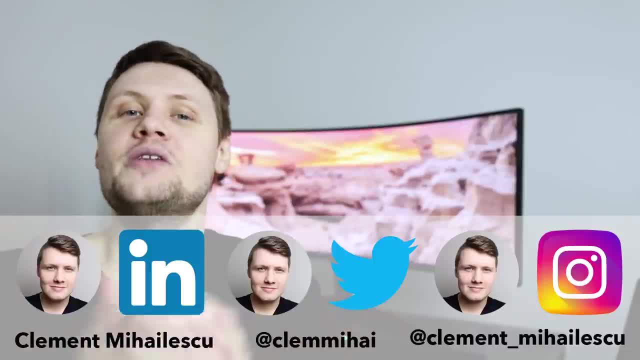 smash the like button. It really helps me out. Subscribe to the channel if you haven't already. Follow me on LinkedIn and Twitter if you enjoy short form written content. Instagram if you like pictures, and otherwise I will see you in the next video.